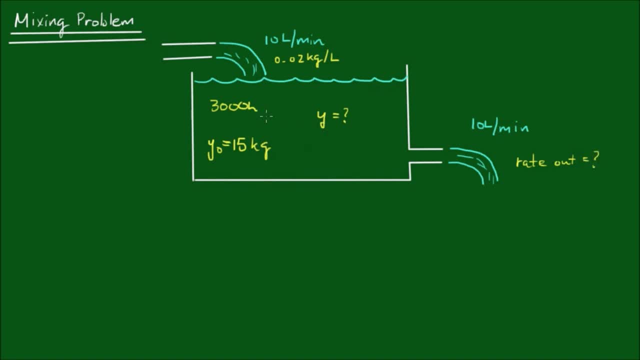 the amount of salt in the tank to increase, But at the same time it's flowing out as well, as the amount of salt that's in the tank is increasing. this quantity Y is also changing over time, right? So we have a rate of change of the quantity dy dt That is also unknown. 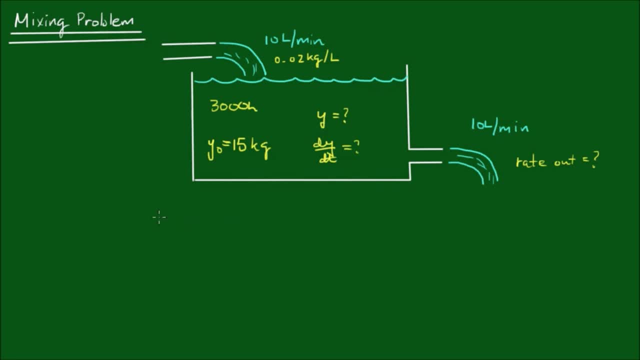 as well. So how do we set this problem up? So let's start with dy, dt, dy on dt. Okay, if we think about it, the rate of change of salt that's in the tank should be equal to the rate that's coming in, minus the rate that's flowing out. And what we do know is the rate. 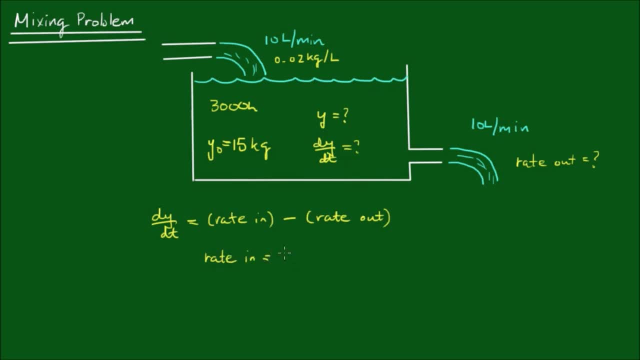 that's coming in. it's equal to 0.02 kilograms or 20 grams per liter. Let's convert that into a flow rate in terms of a mass over time. So we've got 20 kilograms. sorry, 20 grams per liter. 0.02 kilograms per liter by dy dt. 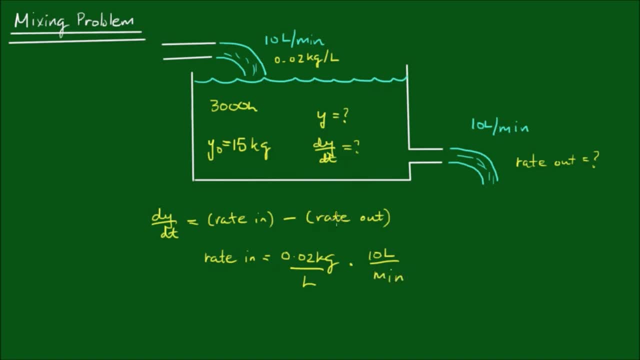 10 liters per minute. So with the units here, the liters cancel out. 0.02 by 10 is equal to 0.2.. So we have 0.2 kilograms per minute coming in. By the same token, the rate out. 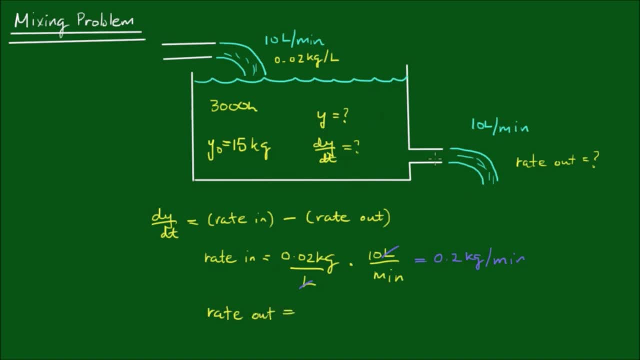 And if we think about it again, the rate out the concentration of solution that's coming out of the tank should be the same as the concentration that's in the tank after it's been mixed properly, right? So we have a quantity y coming out dissolved in 3,000. 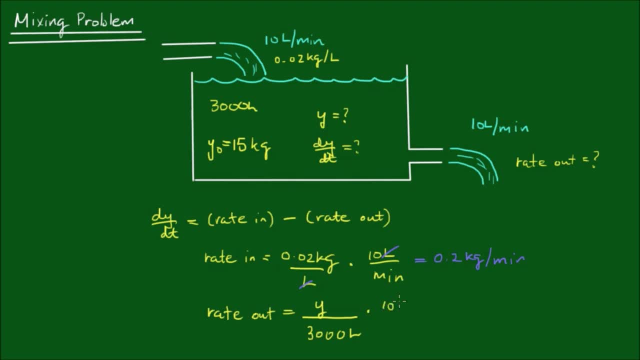 liters, and it's also coming out at a rate of 10 liters per minute. So again, cancel the units. One of the zeros goes from the top and bottom as well, and we have y over 300 kilograms per minute flowing out. So I hope that's starting to make sense. So the 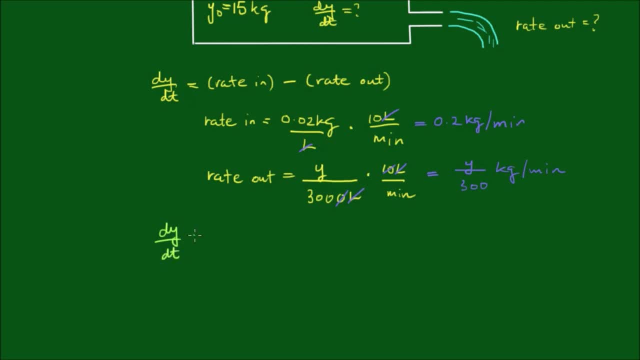 differential equation then becomes: dy on dt is equal to 0.2, I'm going to leave out the units minus y on 300. And if I give this expression on the right a common denominator, we should have 300 by 0.2 minus y, all over. 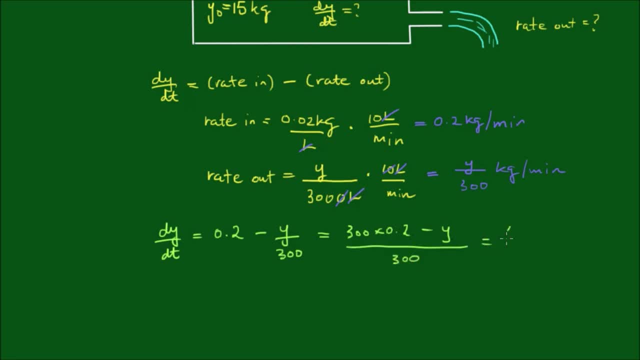 300,, which means we have 60 minus y. Let's call this equation 1.. And equation 1 is my linear first-order differential equation. Okay, so let's take equation 1, and let's get all of the y's on one side onto the right. 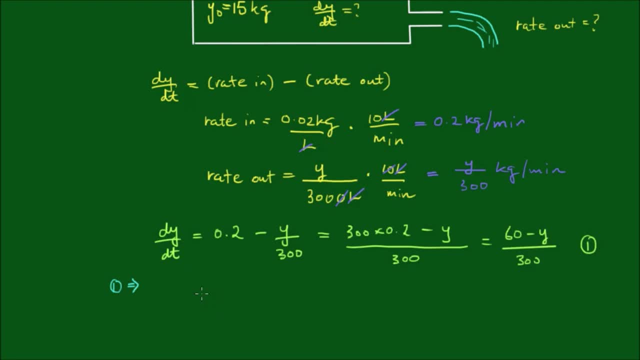 hand side and all of the t's onto the left hand side. So in other words, let's separate the variables. So we have dy on 60 minus y equals dt on 300.. And now the process is to integrate both sides. So the right hand side integrates to. 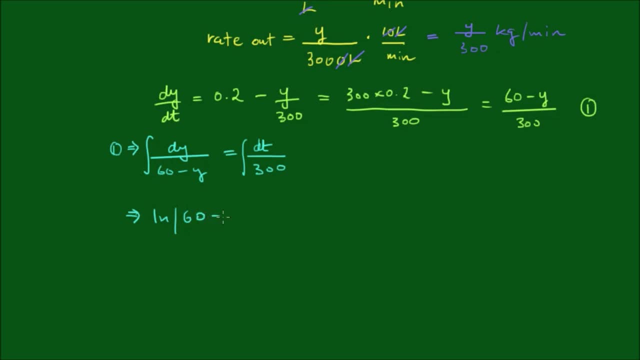 log of 60 minus y And applying the reverse chain rule, we also have to divide by the differentiation of what's in the absolute value bars, and that will be negative 1. And that's equal to 1 on 300 times t plus the integration constant c. Conversely, I could: 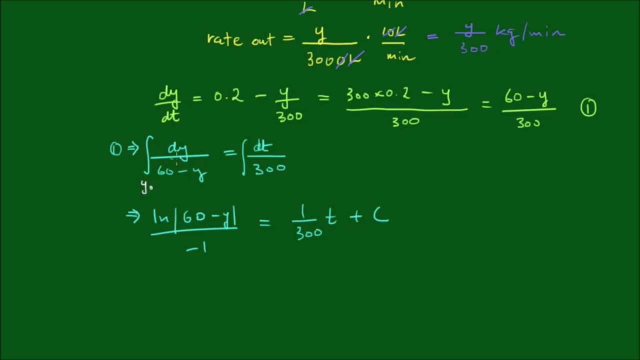 have used definite integrals here, So we are integrating from y0 to y And we're integrating from t equals 0 to t, So it's from 0 to t. But equally I've used an indefinite integral and that's perfectly fine as well. So we have negative of the log of 60 minus y equals t. 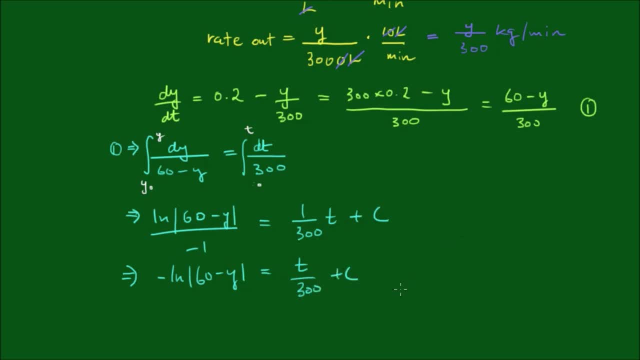 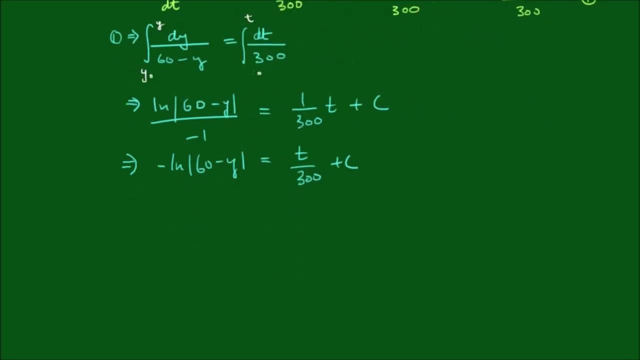 on 300 plus 60 minus y, And the next step is to isolate y so that we can find the quantity as a function of time. I'm going to exponentiate both sides of the equation. So we have e to the negative log of 60 minus y, equals e to the t on 300 plus c. 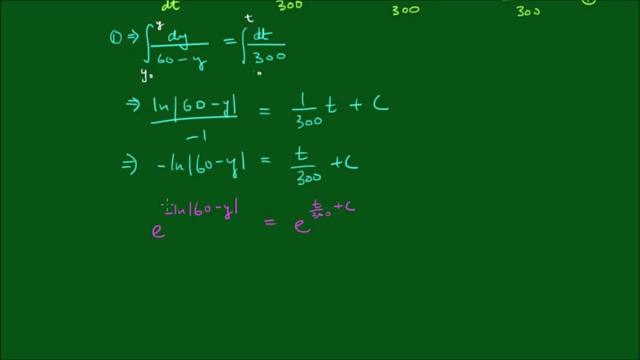 Now one of our log laws of course, is we can take whatever is in front of the logarithm and put it as a power. So I'll write that as e to the log of 60 minus y to the power of negative 1.. And I can write this on the right hand side here as e to the power of t on 300, by e to 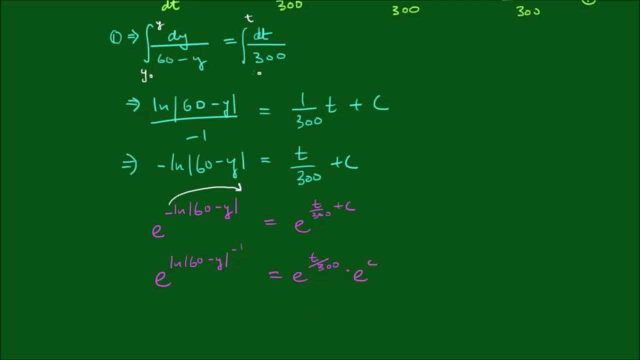 the power of c. So that's just using the addition law of indices. Okay, so the expression on the left hand side simplifies too. These are opposite functions, So we're just left with 60 minus y to the power of negative. 1 is equal to. I'm just 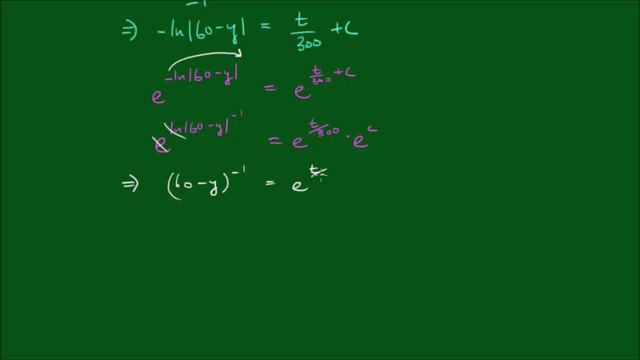 going to keep the right hand side the same for now. So e to the power of t on 300, by e to the power of c, Because now I'm going to apply power of 1 to both sides, power of negative 1 to both. 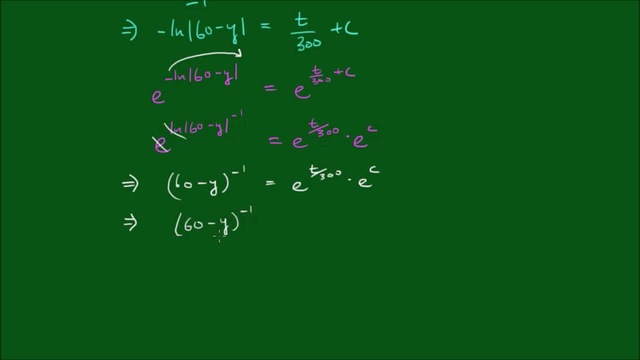 sides, So 60 minus y to the power of negative 1.. And I'm going to raise that again to the power of negative 1 is equal to e to the power of t on 300 by e to the power of c, to the power of negative 1.. 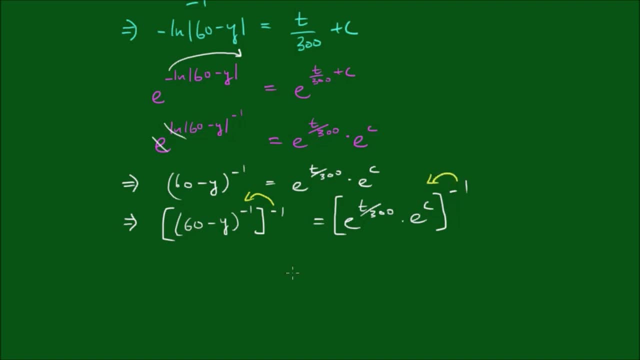 And expanding the powers into the brackets we have, 60 minus y is equal to e to the power of negative t on 300.. Okay, So 60 minus y to the power of negative 1 is equal to e to the power of negative c. 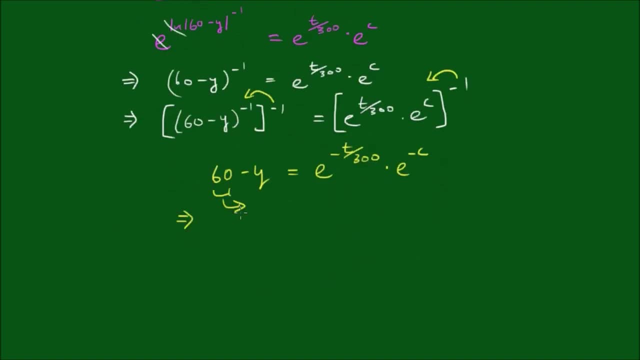 And if we rearrange further, let's take the 60 over to the other side. So negative y equals e to the negative t on 300, by e to the negative c minus 60. And multiplying both sides of the equation by negative 1, we further reduce this to y. 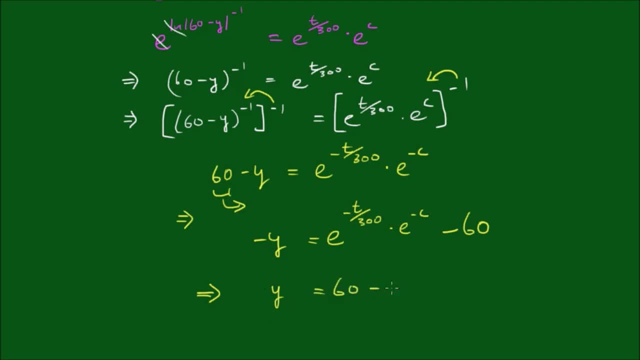 equals positive 60. So 60 minus y to the power of negative 1 is equal to e to the power of negative 1.. And I'm going to write e to the power of negative c as some constant. Let's call that a. 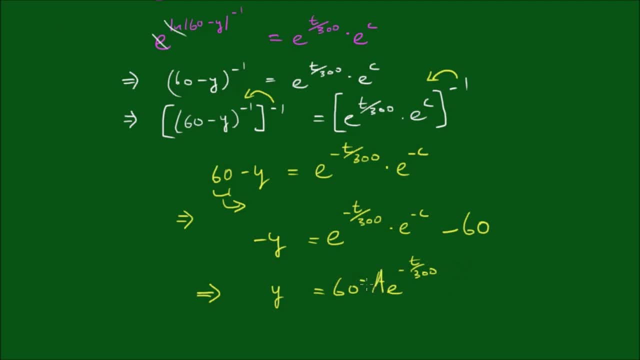 And of course it's prettier to write the a at the front. Okay, So we're nearly done. All that's left to do is to apply the initial condition to find our coefficient a here. So doing that At time equals 0.. 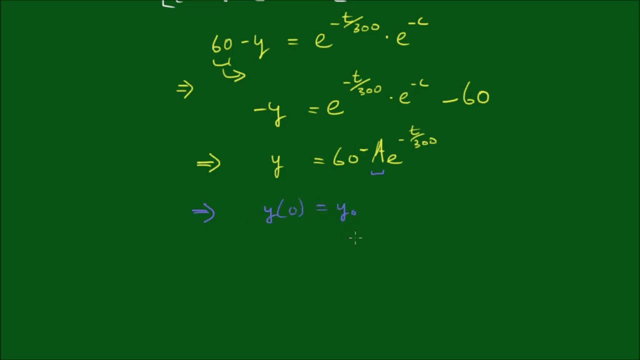 We know we started with the initial amount of salt in the tank, which was 15 kilos, And that's equal to the general expression, which is 60 minus a, by e to the negative 0.. Time equals 0 on 300.. 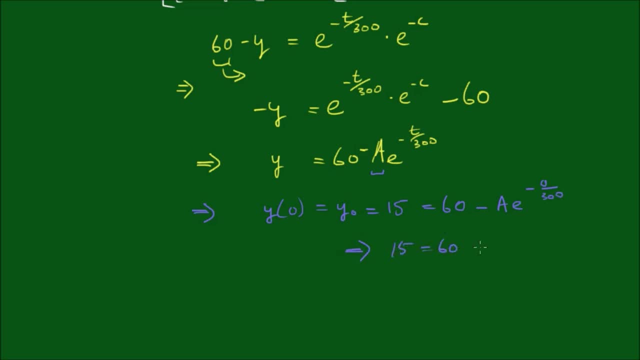 This expression shortens to 15, equals 60 minus a, by e to the 0. And of course Anything to the power of 0 is equal to 1.. So that of course means a is equal to 15.. Sorry, 45.. 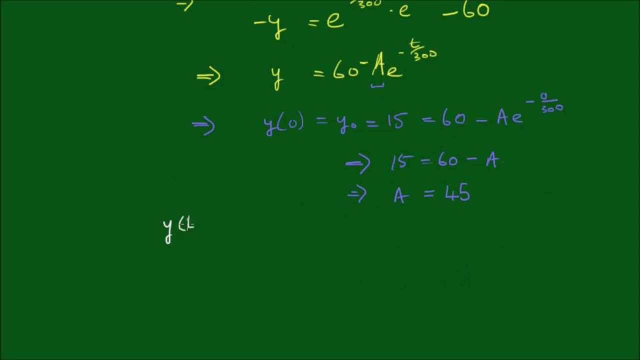 Okay, So problem solved. We have found the expression for the quantity of salt at any given time in the tank. So y of t is equal to 60 minus 15.. Sorry, minus 45.. By e to the power of t. 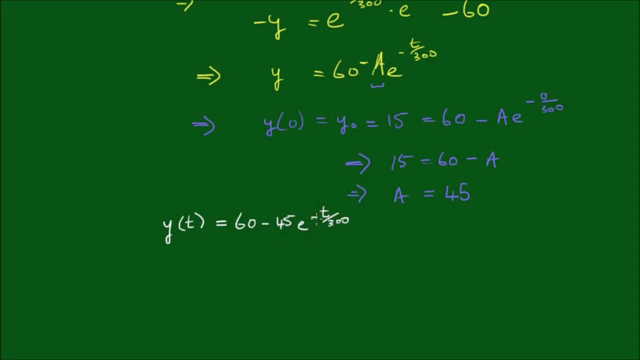 T divided by 300.. E to the power of negative t divided by 300.. All right, So we can plug in any positive value for time And we should be able to precisely determine the amount of salt that's in the tank. Let's see what this solution looks like graphically. 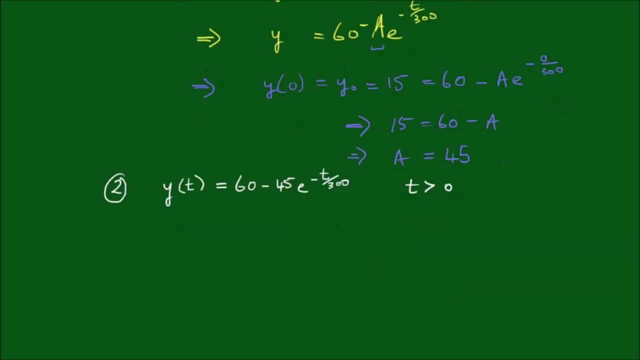 So we'll call this equation 2.. Let's see what equation 2 looks like graphically. Okay, So here's a graph that I prepared earlier. So, as we can see, The initial level of salt that's in the tank Is 15,, 15 kilos, 15 kilograms. 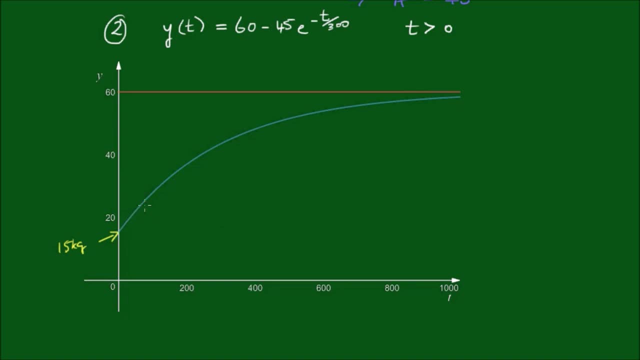 As the solution starts pouring in, We can see that there's quite a relatively rapid increase in the solution: Increase in the quantity, rather of salt, for the first 400 minutes, Roughly the first 7 hours, But, as we can see, over a sufficiently long time. 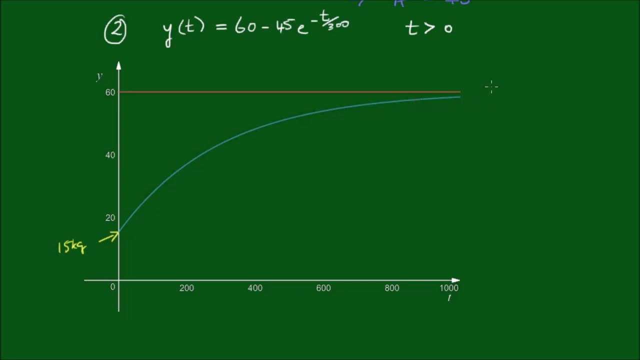 The amount of salt that's in the tank Tapers towards 60 kilograms. So it seems we'll never exceed 60 kilograms of salt in the tank, Simply by virtue that there is an outflow of the brine at the same rate that it's coming. 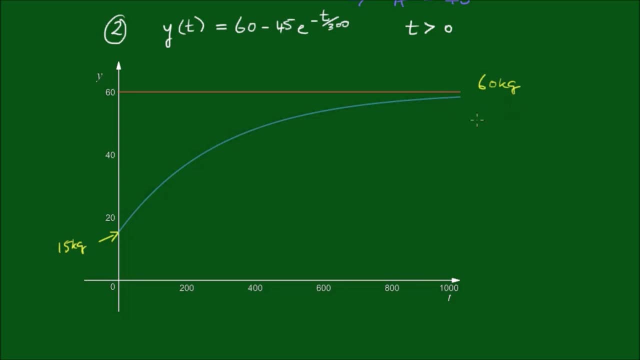 in, So we'll reach a steady state solution in the tank And a steady state quantity of 60 kilos. Okay, so that's our mixing problem done. If you have any questions, feel free to ask in the comments below If I haven't made anything clear.